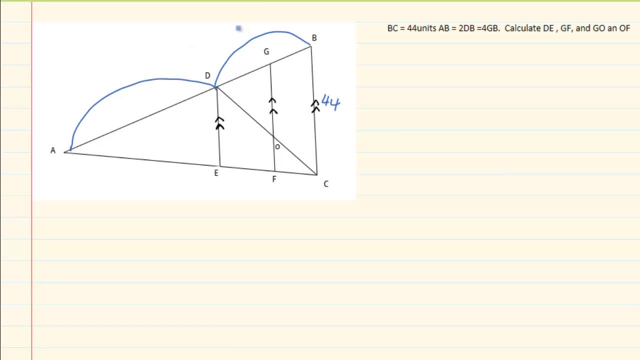 that AB is 2 of DB, then it means that this side is equal, creating a similar ratio. So if you look at the triangle, I have a similar ratio. Now, if you look at that immediately, you should say: but if I have a parallel line and I have same sign, then that means it's. 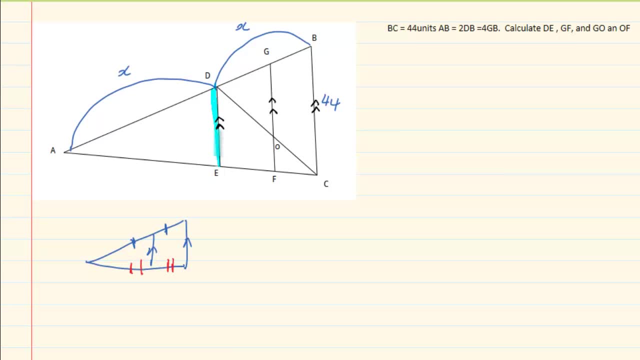 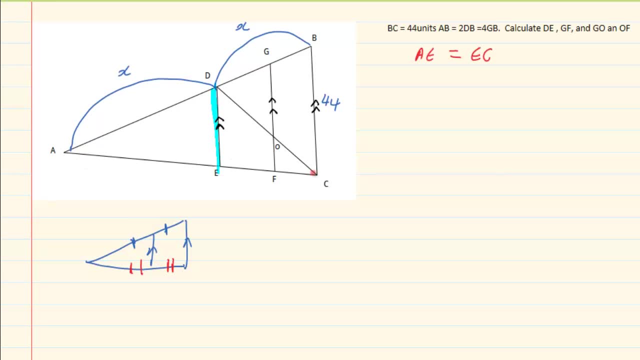 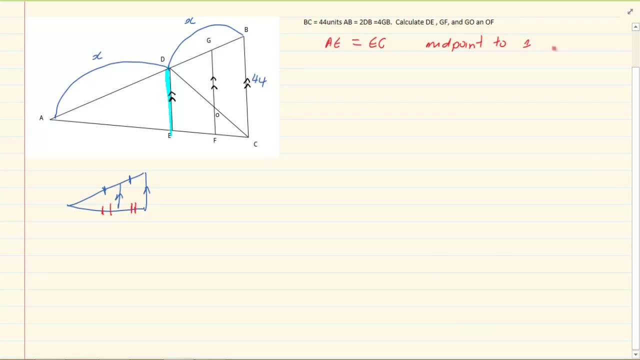 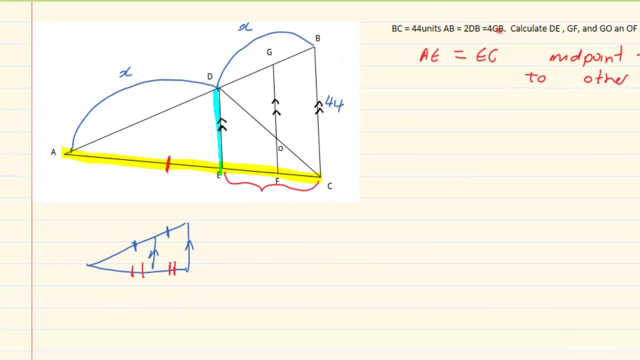 I will be able to say that AE is equal to EC, and the reason is: midpoint to one side and parallel to another. So I do have now that AE is equal to EF Let's talk about then. it says that 2db is equal to 4gb. 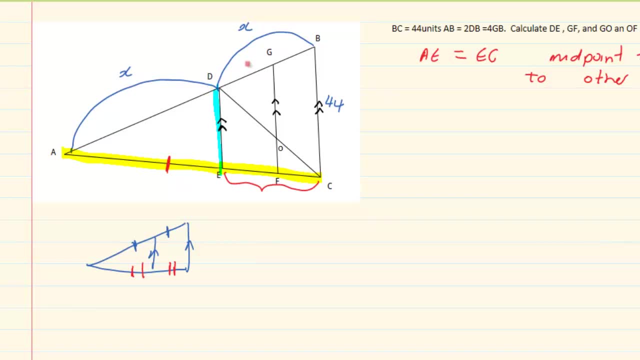 Now that means if I take 2db, 2 of this, it's equal to 4 of gb. They are telling us that gb is equal to dg. So again, we've got the same concept. If you're looking now at the different triangles that are available to us, 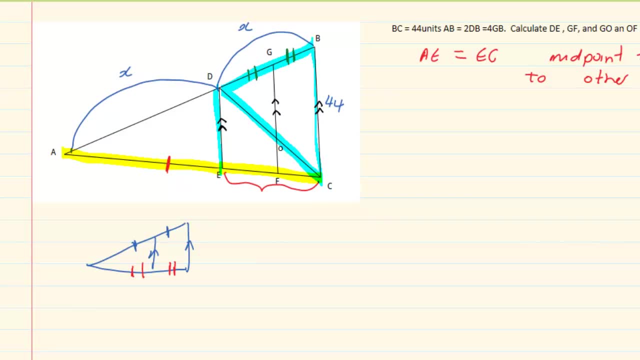 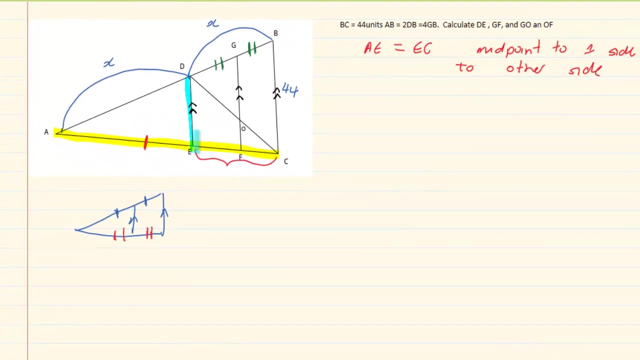 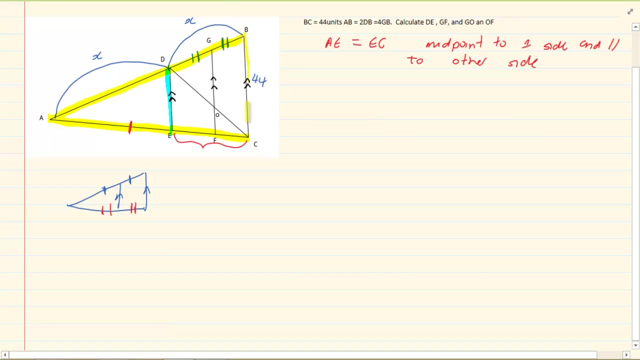 you'd be able to see the same rule. Now let's go on to the question. They're asking us to calculate de. Now, if you're looking at the triangle, let us look at the yellow triangle. So we're ignoring everything else. 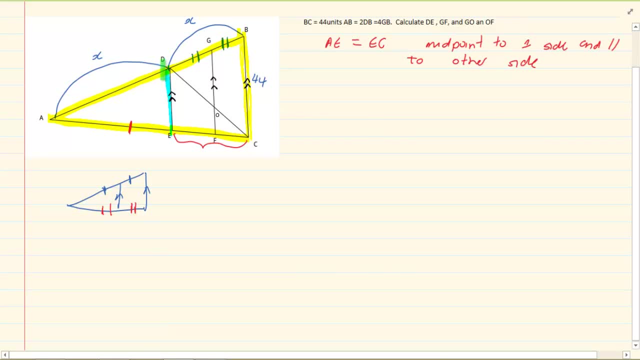 If you look at the yellow triangle, we have that db and ad are equal, and we've got that ae is equal to ec. We've also got that they are parallel. So what's the difference? So what's the difference? 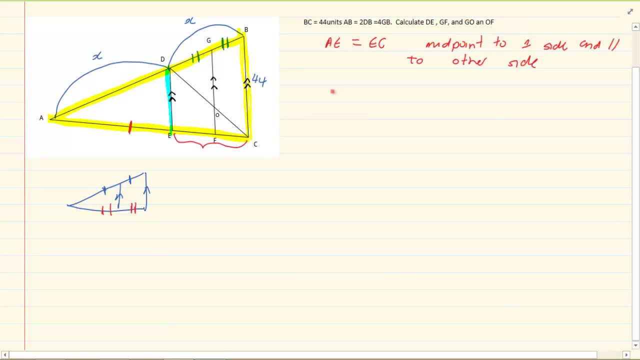 So what can we say about de and bc? De is going to equal to a half of bc, And why? We know it's the midpoint theorem. The theorem states: if I have two sides that are equal, so we're looking at the x, remember? 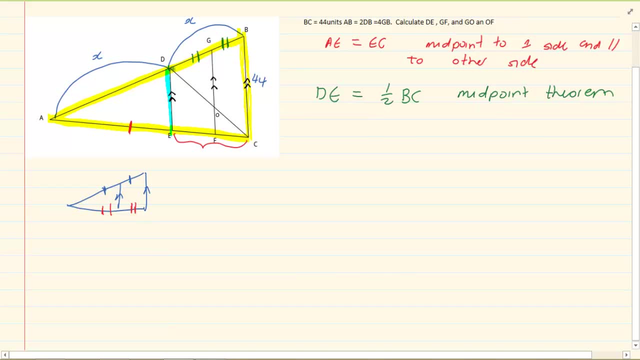 So that's the midpoint and the opposite side is also the midpoint. Then the lines are parallel, which is also given. Then it is half, So de is going to equal to a half of 44,, which is going to equal to 22.. 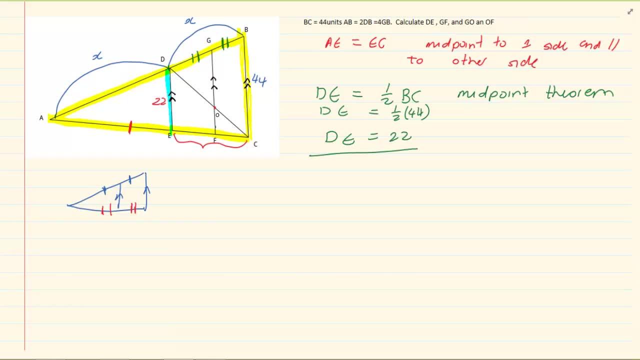 de is equal to 22.. Now they're asking us to calculate gf. But gf, you can't say, hey, I'm using the triangle gfa, Because, look, this side is not equal to this side. Neither is dg equal to ga. 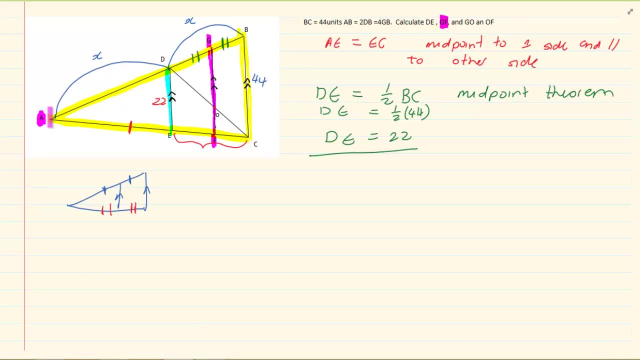 So we can't use the rule where we can say, hey, you know what, it's, just half, and let me take it. We have to look for triangles that will actually apply that rule. Now let's take the specific triangle. 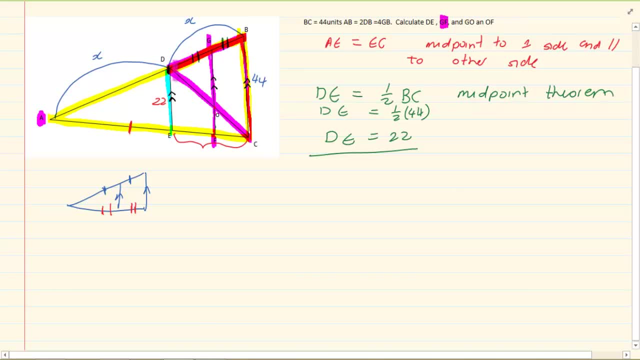 If we take that triangle, we know that gb is equal to dg because it was given to us. We also know that bc is parallel to go. So what we can say is that go is equal to a half of bc. Why is it equal to a half of bc? 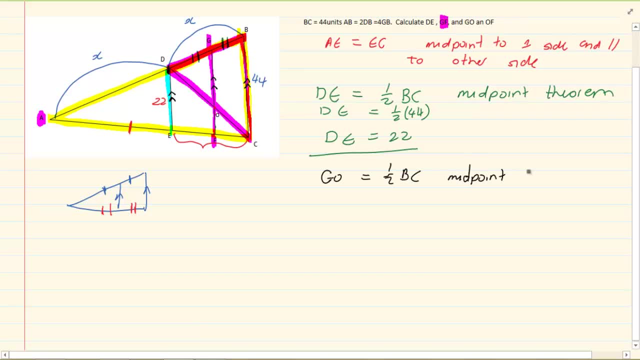 Because we've got midpoint to one side and parallel to another. So you must understand which triangle I'm working with. I'm working with b, d, c. I know they're parallel And I know they're equal. So you must be able to understand which triangle I'm working with. 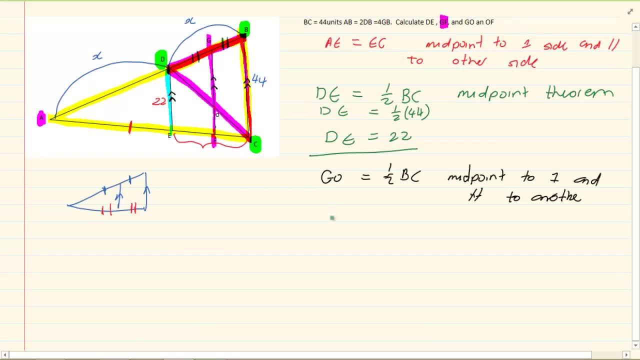 Now that gives me the length of go, So I have that go is going to equal to a half of 44, which is equal to 22.. But that is not answering my question, because now I've got a piece but I don't have the other piece. 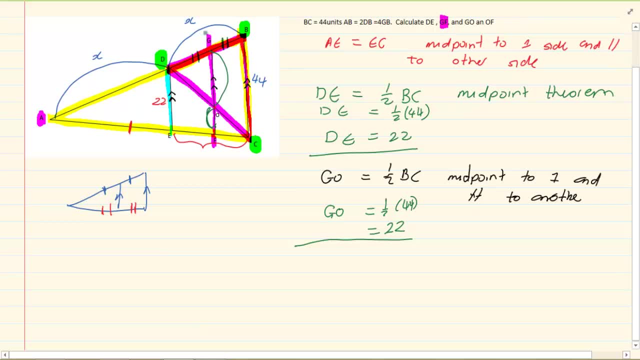 Now, if we've proven that b, c, d is a midpoint theorem, then I can say that do is equal to oc, do is equal to oc And our reason is: midpoint to one side parallel to another. If that is equal. 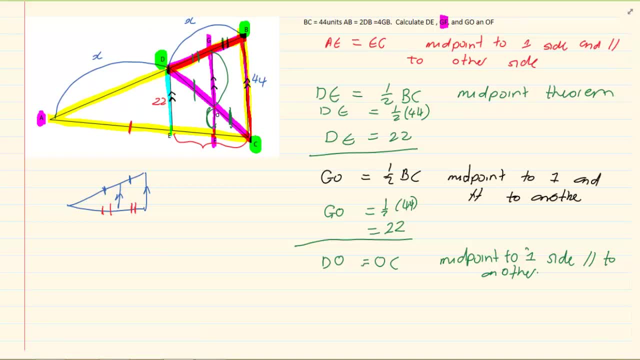 then I know that. look, pay attention to which triangle I'm using now. Now I'm going to use this triangle Now I have that. it's parallel. I've got that. d e is parallel to g f. That was given. 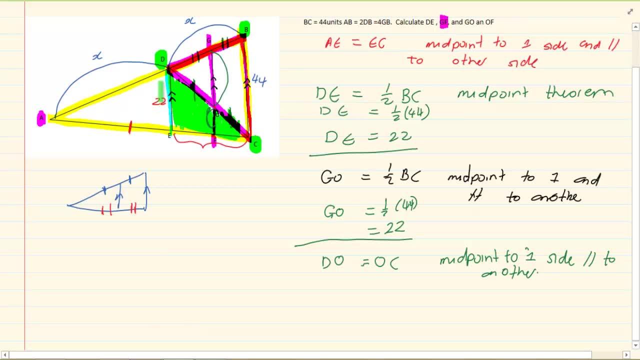 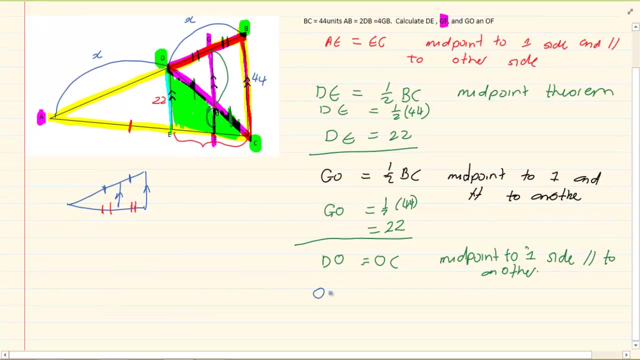 So since they're parallel- and I have that they are midpoints- I can say that of of is equal to a half of d? e. What you need to notice is that we're working with the triangle upside down. now. 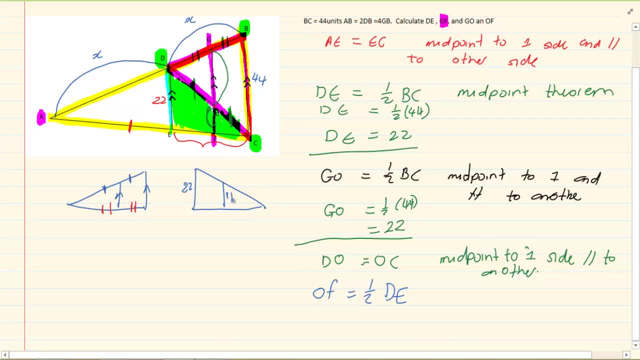 I'm working here, I've got 22, and I'm working here, So you're working with the triangle upside down. So we have that of is equal to a half of d e. Now our reason is still midpoint to one side. 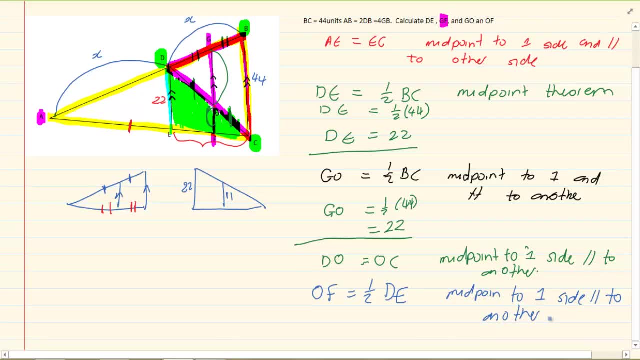 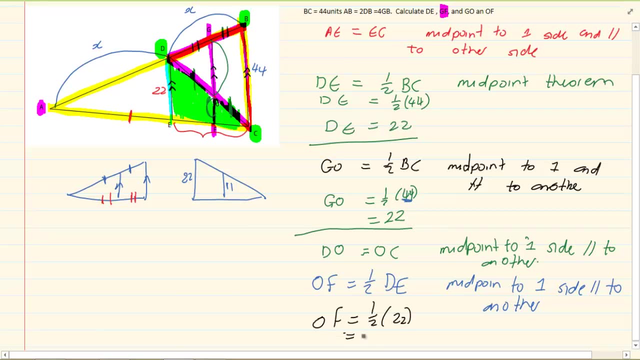 parallel to another. So we've got of is going to equal to a half times 22,, which is going to equal to 11.. So what is the final length of g f? g f is going to equal to g o plus o f. 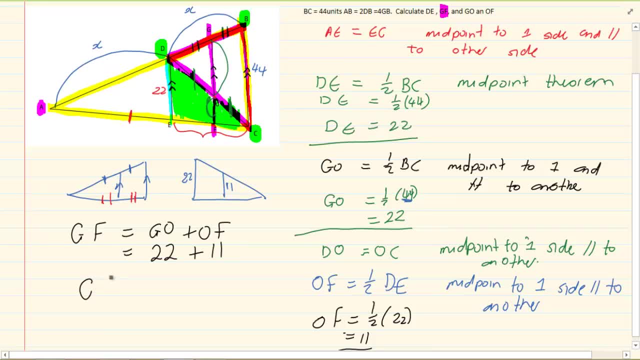 g o is 22.. o f is 11.. So the final length of g f is going to be 33 units. Okay, Now, if you continue, they say: calculate the length of g o, which we've already done. 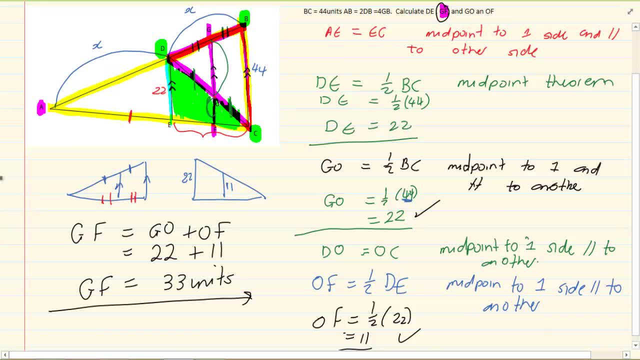 and calculate the length of o- f. Now we've answered all the questions. There is g, f and the very first one was d- e. Thank you for watching.